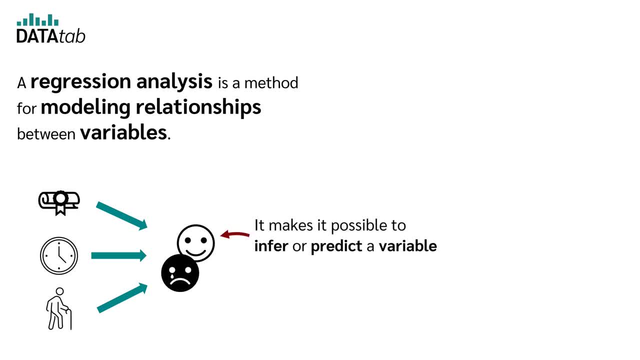 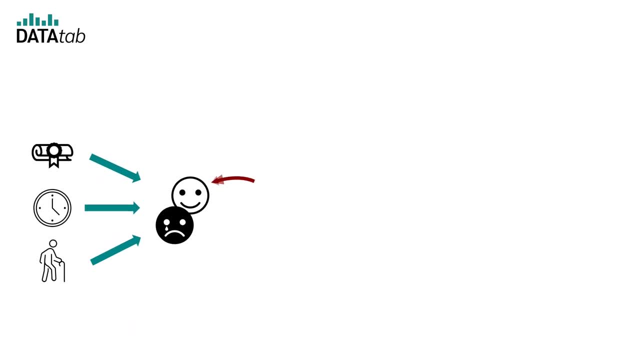 relationships between variables. It makes it possible to infer or predict a variable based on one or more other variables. The variable we want to infer or predict is called a dependent variable or criterion. The variables we use for prediction are called independent variables or predictors. But what is the difference between a linear regression and a logistic? 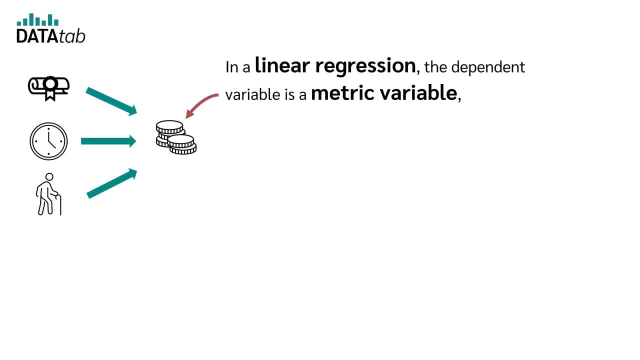 regression. In a linear regression, the dependent variable is a metric variable, for example salary or electricity consumption. In a logistic regression, the dependent variable is a dichotomous variable. What is a dichotomous variable? Dichotomous variables are variables with. 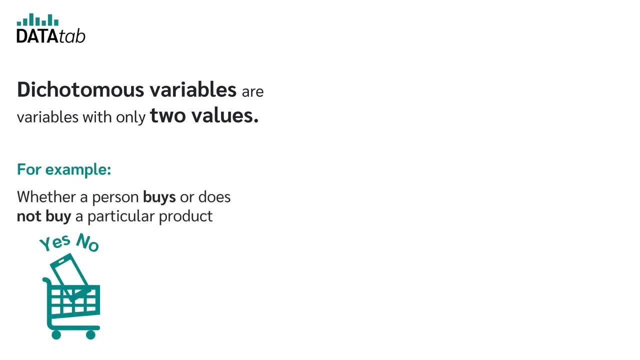 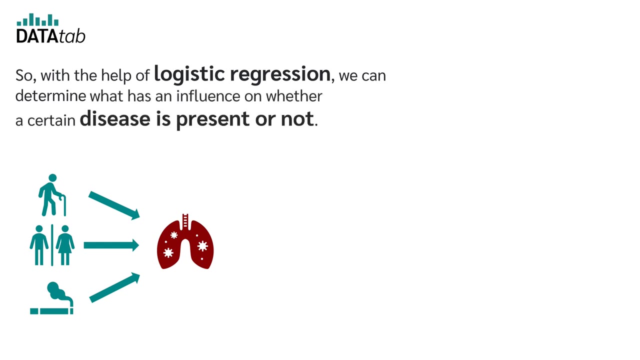 only two values, For example, whether a person buys or does not buy a particular product, or whether a disease is present or not. So with the help of a logistic regression, we can determine what has an influence on whether a certain disease is present or not. 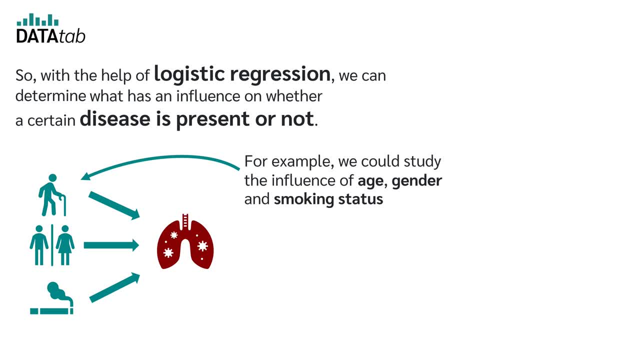 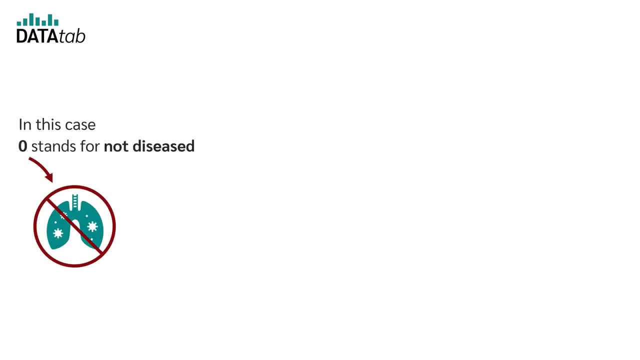 For example, we could study the influence of age, gender and smoking status on that particular disease. In this case, 0 stands for not deceased and 1 for deceased, and the probability for the occurrence of the characteristic 1, characteristic present is estimated. 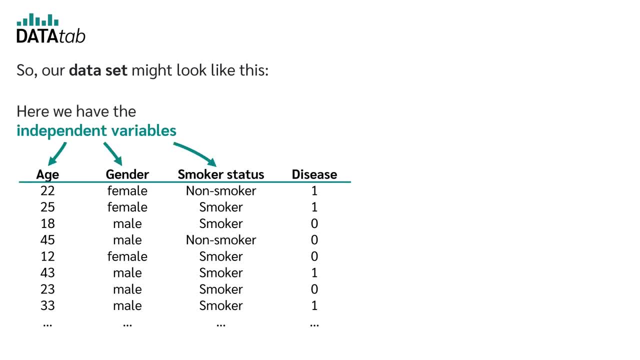 So our dataset might look like this: Here we have the independent variables- age, gender, smoker status and here the dependent variable with 0 and 1.. We could now investigate what influence the independent variables have on the disease. If there is an influence, then 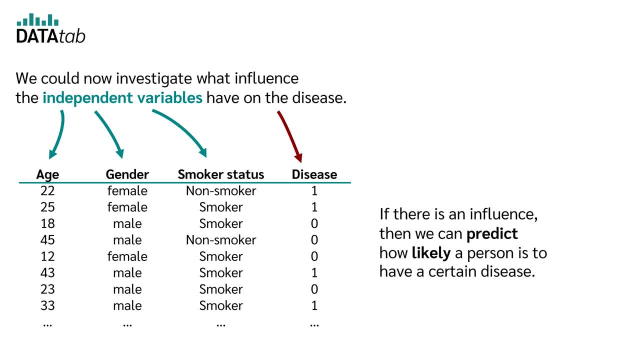 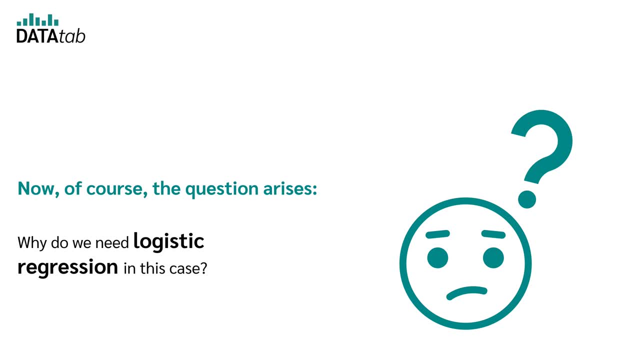 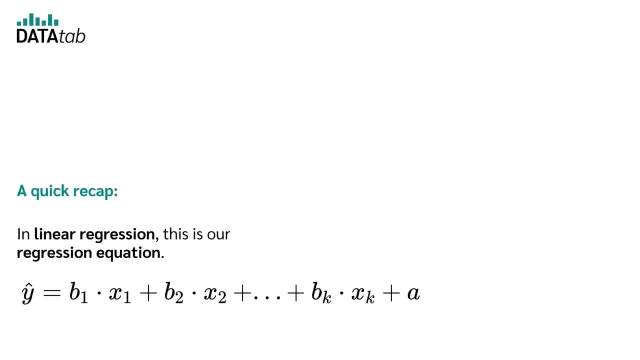 we can predict how likely a person is to have a certain disease. Now, of course, the question arises: Why do we need logistic regression in this case? Why can't we just use linear regression? A quick recap: In linear regression- this is our regression equation- We have the dependent. 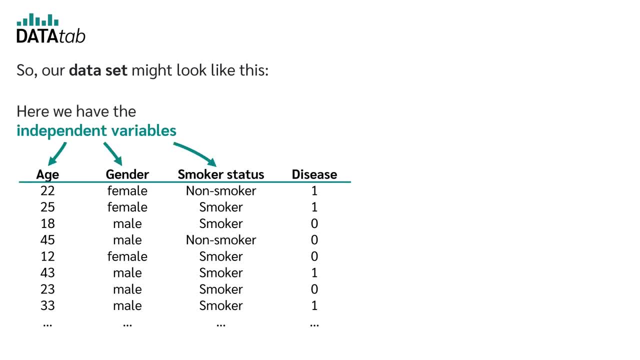 So our dataset might look like this: Here we have the independent variables- age, gender, smoking status and here the dependent variable with 0 and 1.. We could now investigate what influence the independent variables have on the disease. If there is an influence, then 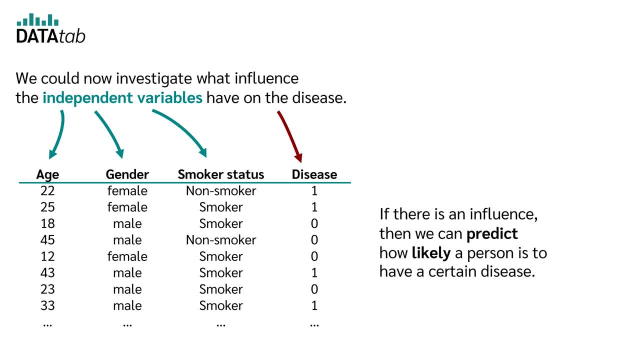 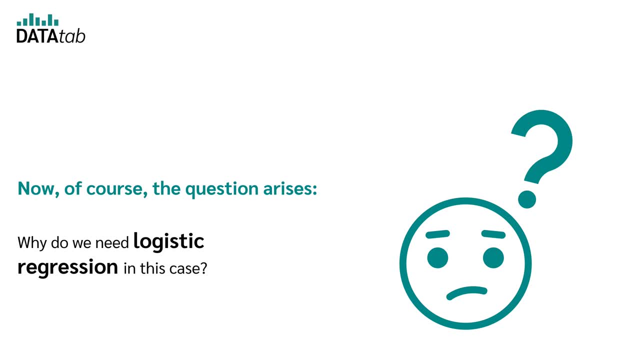 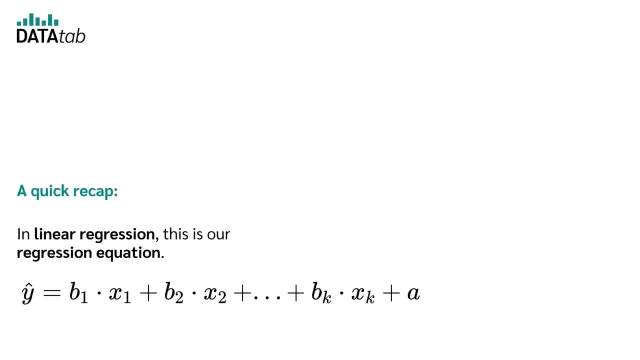 we can predict how likely a person is to have a certain disease. Now, of course, the question arises: Why do we need logistic regression in this case? Why can't we just use linear regression? A quick recap: In linear regression- this is our regression equation- We have the dependent. 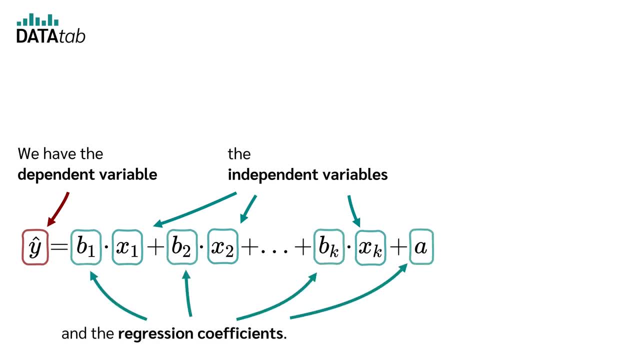 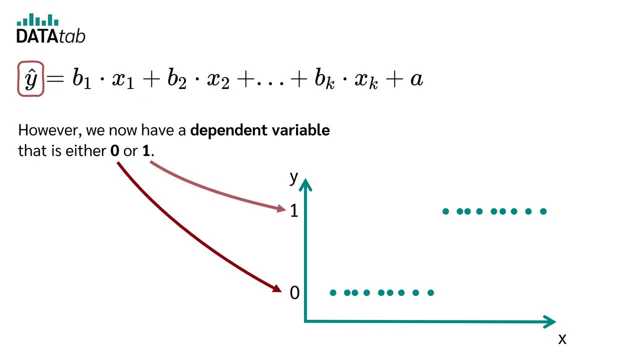 variable, the independent variables and the regression coefficients. However, we now have a dependent variable that is either 0 or 1. No matter which value we have for the independent variables- only 0 or 1.. A linear regression would now simply put a straight line through the points We can. 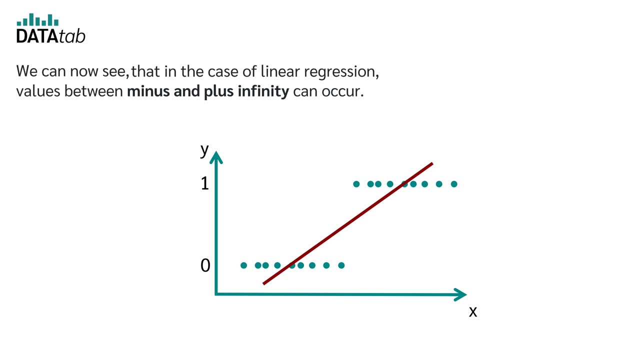 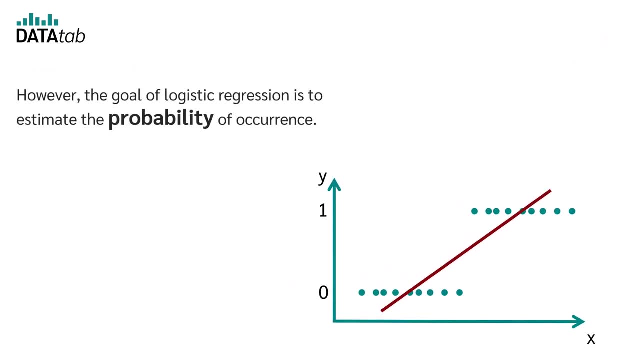 now see that in the case of linear regression, values between minus and plus, infinity can occur. However, the goal of logistic regression is to estimate the probability of occurrence. The value range for the prediction should therefore be between 0 and 1.. So we need a. 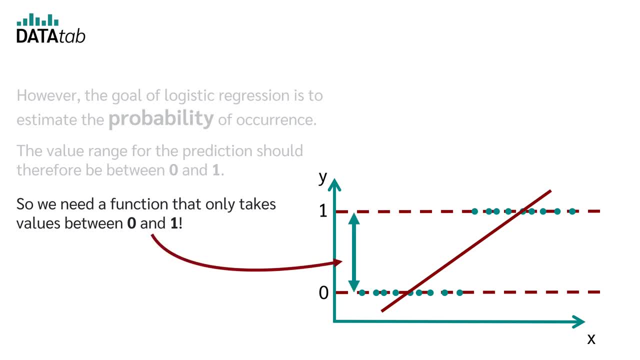 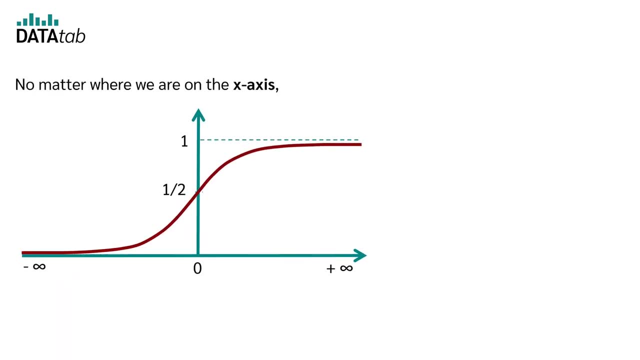 function that only takes values between 0 and 1.. And that is exactly what the logistic function does, No matter where we are on the x-axis, between minus and plus infinity, only values between 0 and 1 result, And that is exactly what we want. 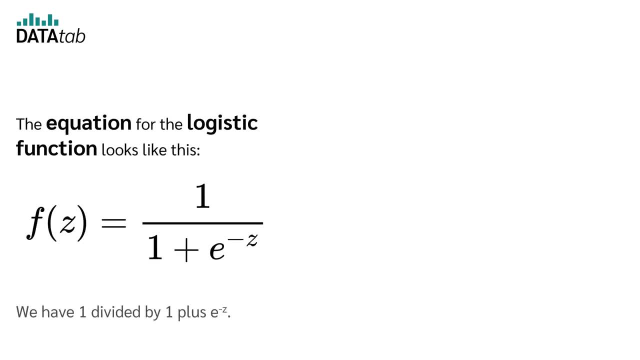 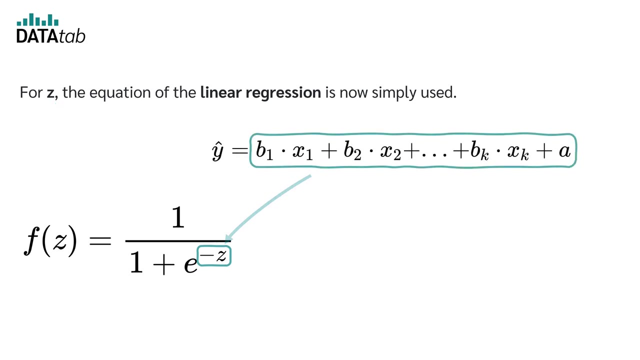 The equation for the logistic function looks like this: We have 1 divided by 1 plus e to the power minus z. Logistic regression now uses the logistic function For z. the equation of the linear regression is now simply used. This gives us this equation: 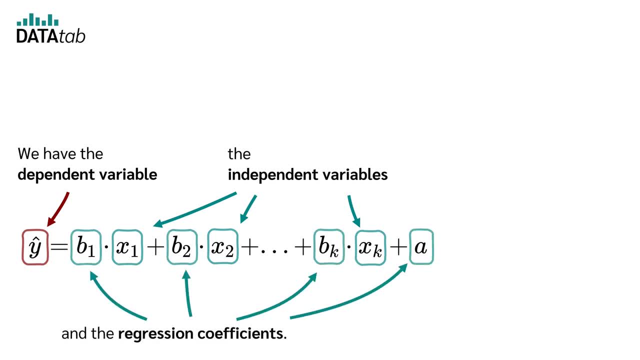 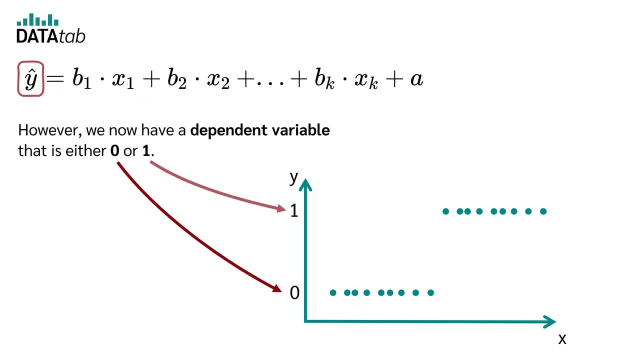 variable, the independent variables and the regression coefficients. However, we now have a dependent variable that is either 0 or 1.. No matter which value we have for the independent variables, only 0 or 1 results. A linear regression would now simply put a straight line through the points We can. 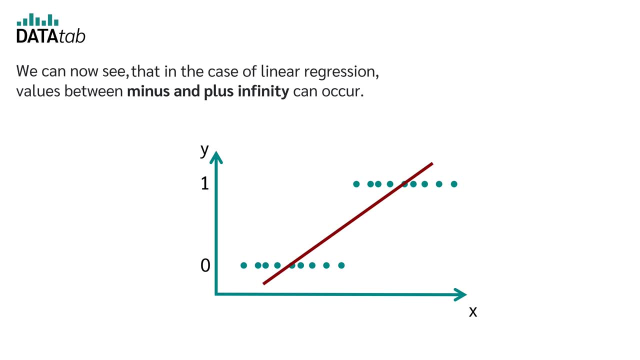 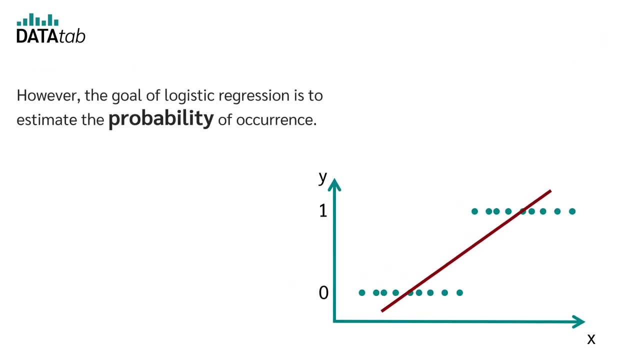 now see that in the case of linear regression, values between minus and plus infinity can occur. However, the goal of logistic regression is to estimate the probability of occurrence. The value range for the prediction should therefore be between 0 and 1.. So we need a function that only takes values between 0 and 1.. And that is exactly what. 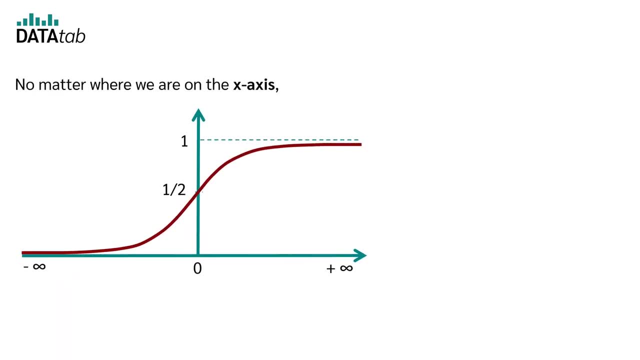 the logistic function does No matter where we are on the x-axis between minus and plus. infinity, only values between 0 and 1 result, And that is exactly what we want. The equation for the logistic function looks like this: We have 1 divided by 1 plus e. 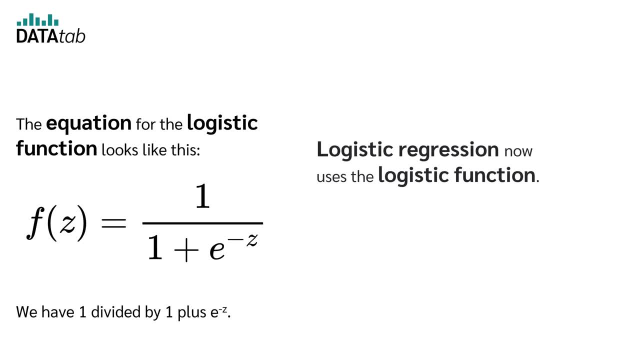 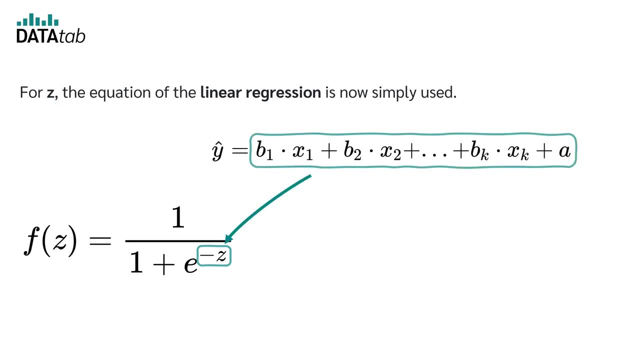 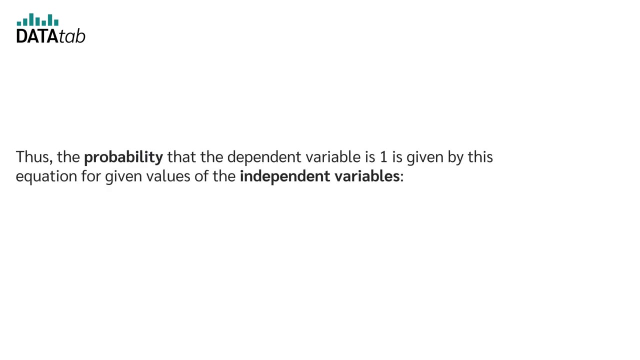 to the power of minus z. Logistic regression now uses the logistic function For z. the equation of the linear regression is now simply used. This gives us this equation. Thus the probability that the dependent variable is 1 is given by this equation for given values. 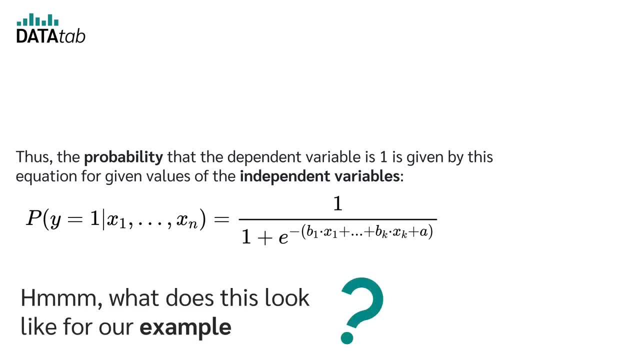 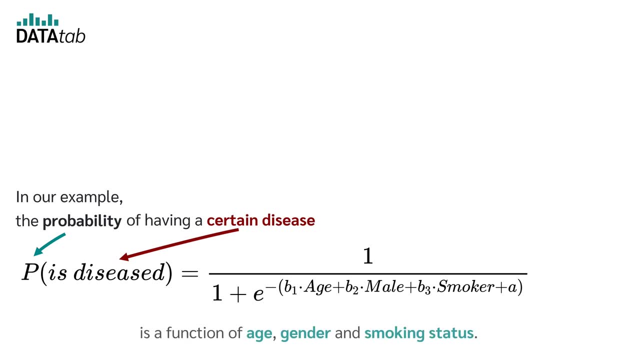 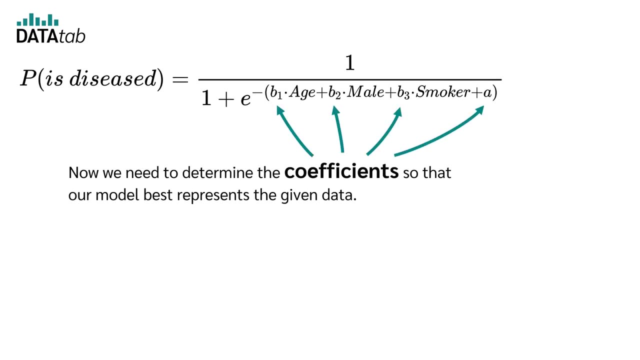 of the independent variables. Hmm, what does this look like for our example? In our example, the probability of having a certain disease is a function of age, gender and smoking status. Now we need to determine the coefficient so that our model best represents the given data. 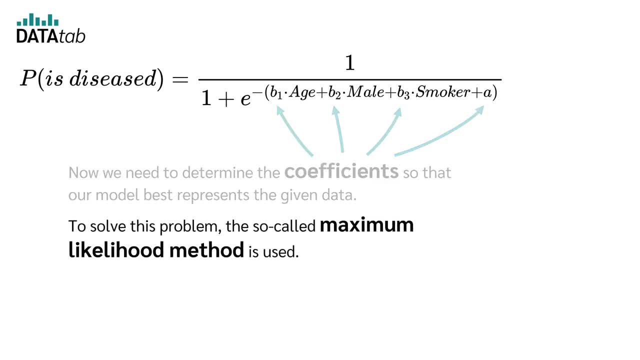 To solve this problem. the so called Maximum Likelihood Method is used For this purpose. there are good numerical methods that can solve the problem efficiently. A statistics program such as SQL sends methods to the information as calculated in pure DataDap. therefore calculates the coefficients b1, b2 to bk and a. 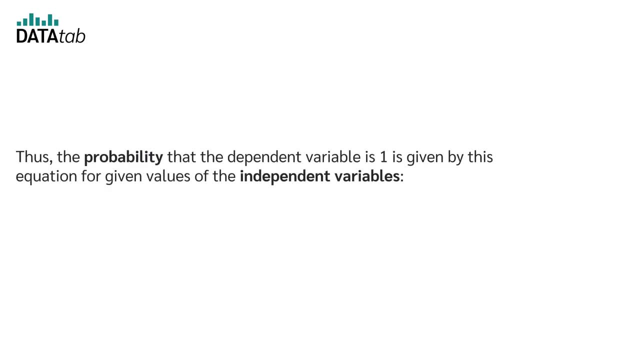 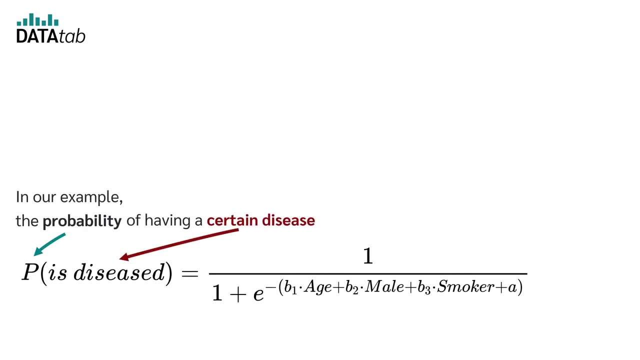 Thus, the probability that the dependent variable is 1 is given by this equation for given values of the independent variables. Hmm, what does this look like for our example 1. ± 1.. For example, the probability of having a certain disease is a function of age, gender and smoking. 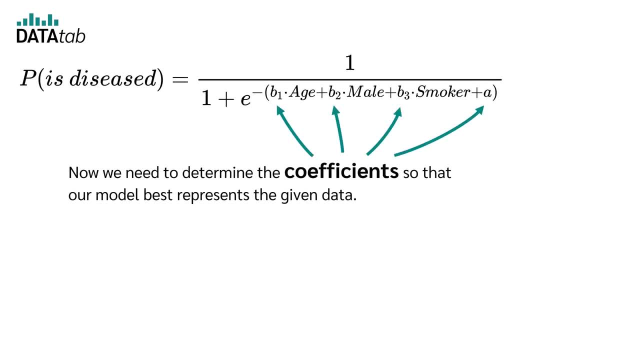 status. Now we need to determine the coefficient so that our model best represents the given data. To solve this problem, the so-called maximum likelihood method is used For this purpose. there are good numerical methods that can solve the problem efficiently. A statistics program such as DataDap therefore calculates the coefficients b1, b2 to bk and 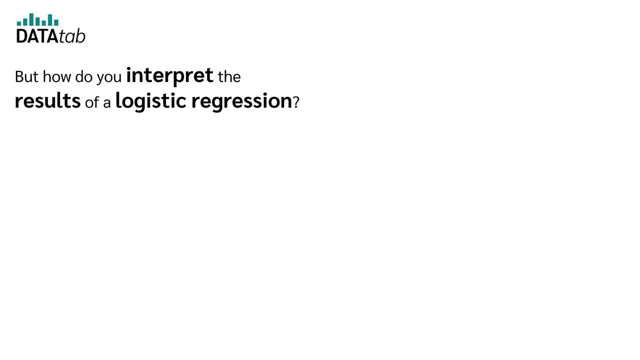 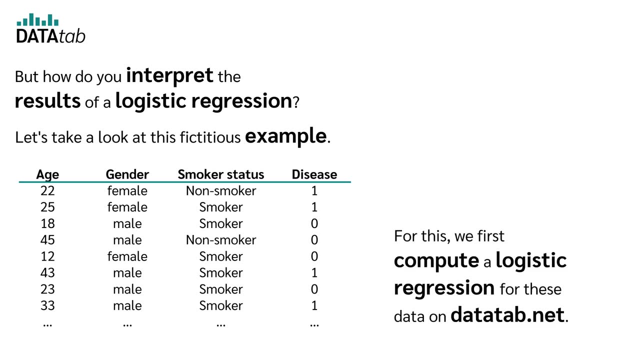 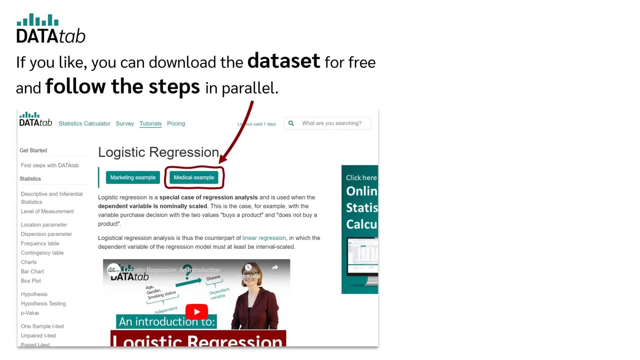 a, But how do you interpret the results of a logistic regression? Let's take a look at this fictitious example. For this, we first compute a logistic regression for these data on DataDapnet. If you like, you can download the dataset for free and follow the steps in parallel. 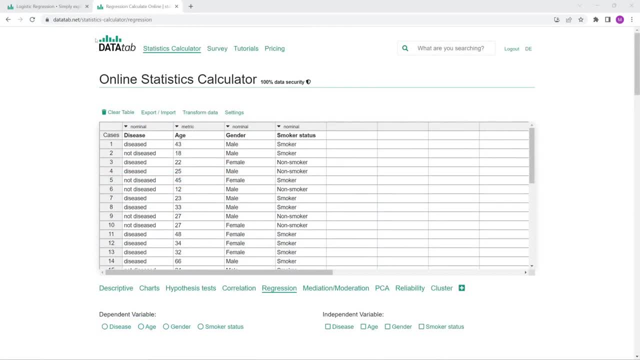 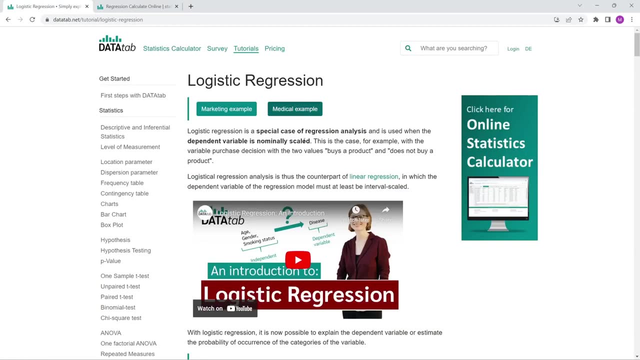 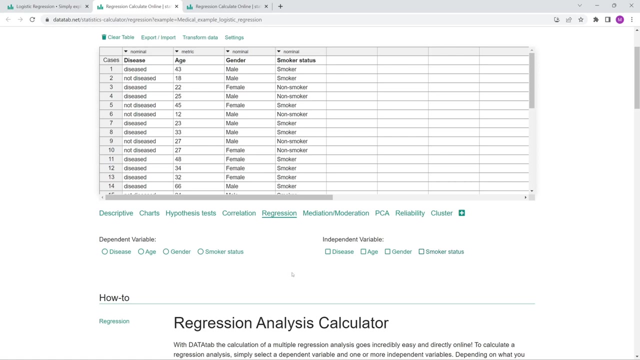 You can find the link in the video description. We go to DataDapnet and copy our own data into this table. I just already loaded the dataset from the link. When we copy our data in here, the variables show up down there. 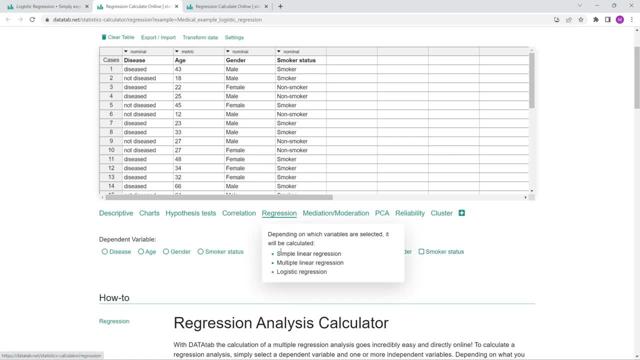 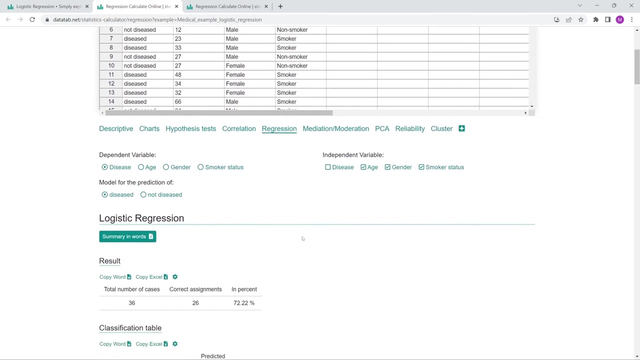 We want to calculate a logistic regression, so we just click on Regression. Depending on how our dependent variable is scaled, DataDap will calculate a logistic regression. We can calculate either a logistic or a linear regression. under the tab Regression, We choose disease as the dependent variable and age, gender and smoking status as the 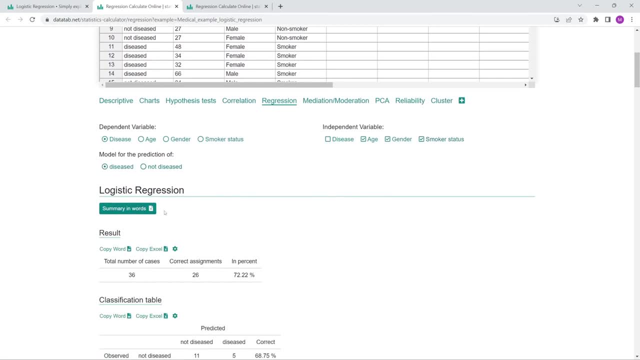 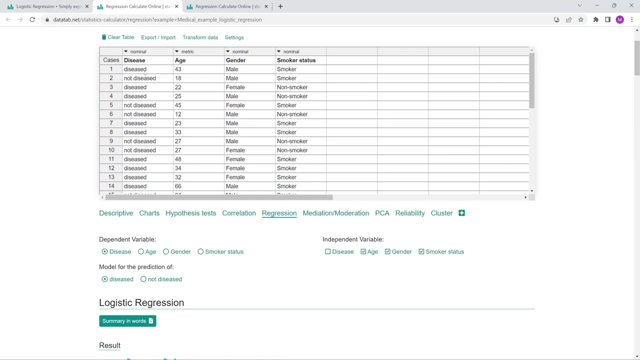 independent variables. DataDap now calculates a logistic regression for us. Now we can choose for which category we want to build the regression model. Our data could also look like this: That there is not not disease, Not deceased and deceased, but zero and one. 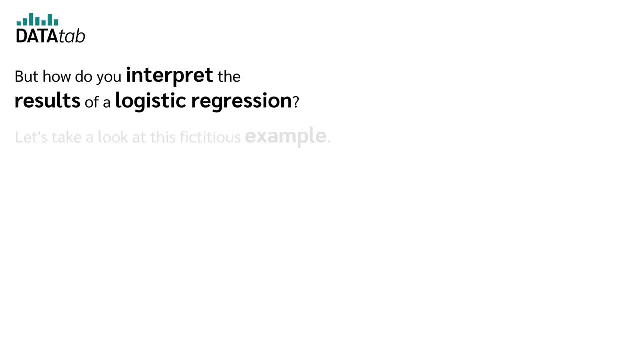 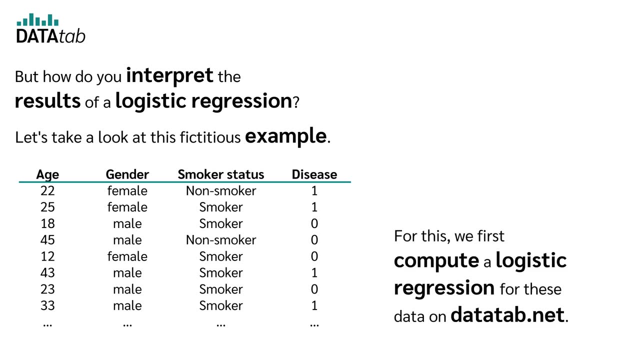 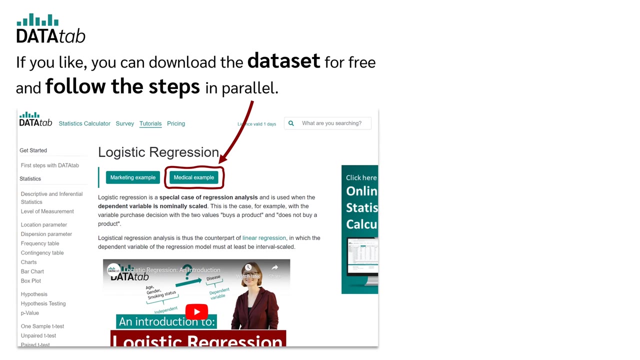 But how do you interpret the results of a logistic regression? Let's take a look at this fictitious example. For this, we first compute a logistic regression for these data on DataDapnet. If you like, you can download the dataset for free and follow the steps in parallel. 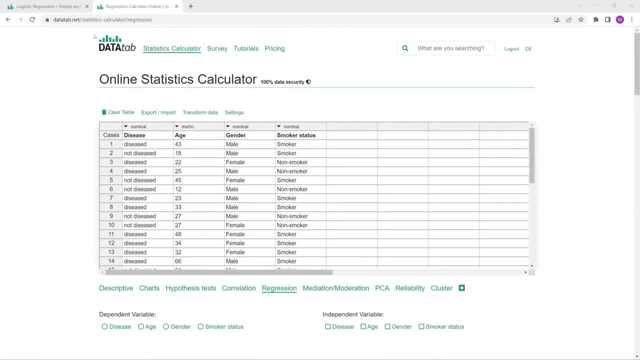 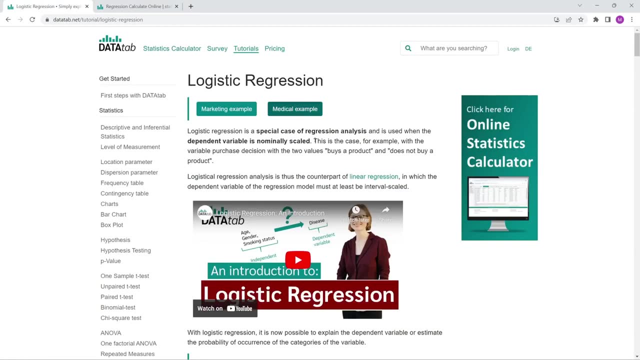 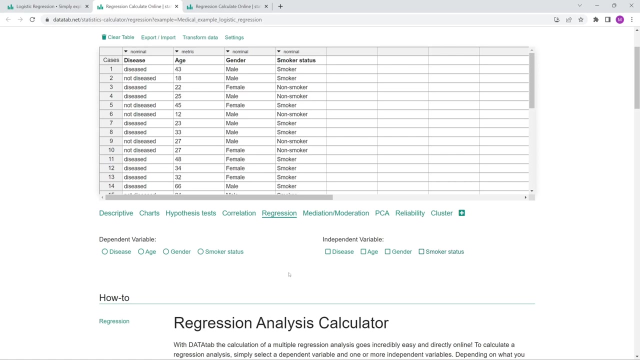 You can find the link in the video description. We go to DataDapnet and copy our own data into this table. I just already loaded the dataset from the link. When we copy our data in here, the variables show up down there. 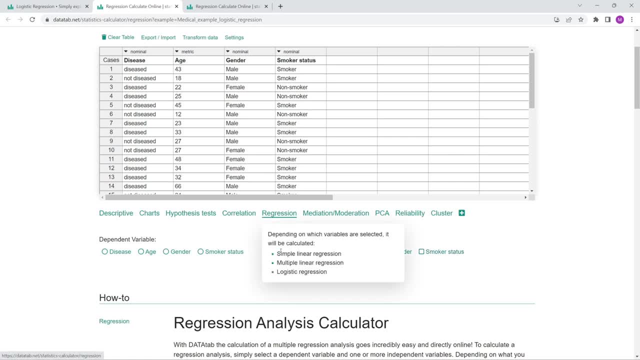 We want to calculate a logistic regression, so we just click on Regression. Depending on how our dependent variable is scaled, DataDap will calculate a logistic regression, So we just click on Regression. We can also calculate either a logistic or a linear regression under the tab Regression. 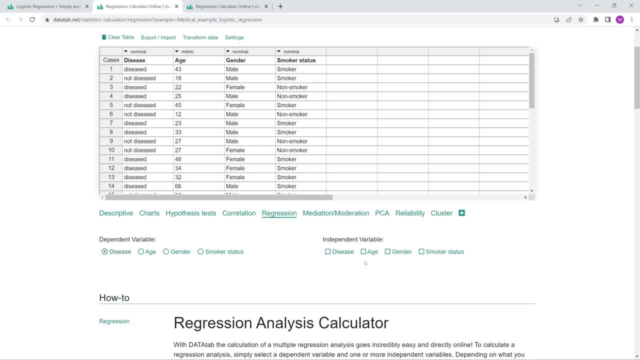 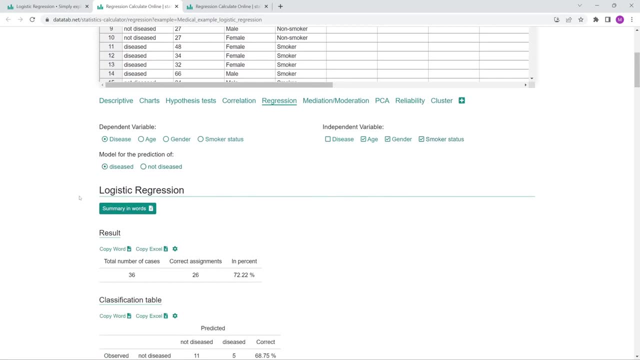 We choose disease as the dependent variable and age, gender and smoking status as the independent variables. DataDap now calculates a logistic regression for us. Now we can choose for which category we want to build the regression model. Our data could also look like this: 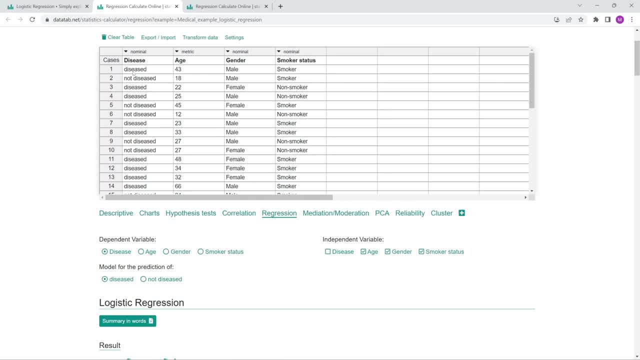 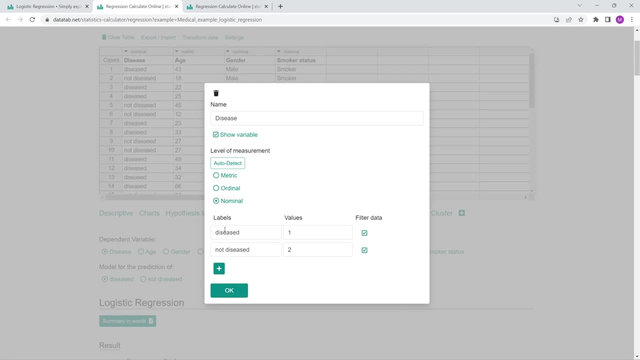 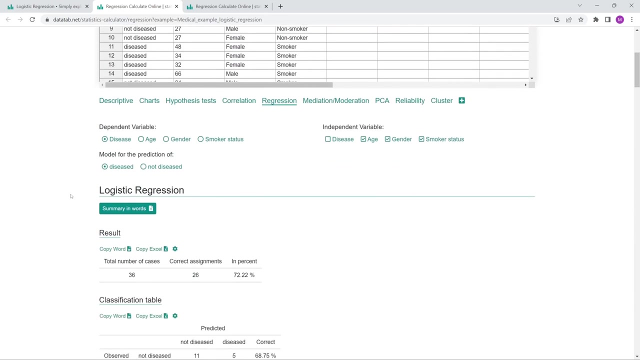 That there is not not disease, Disease and disease, but 0 and 1. Then we would just need to click here and enter the labels: One is diseased and zero is not diseased. Before we go into detail about the different results, a little tip. 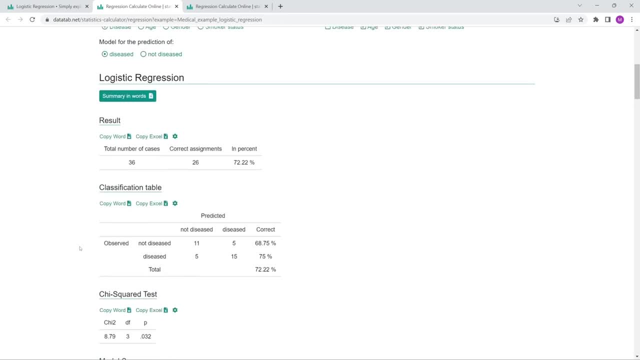 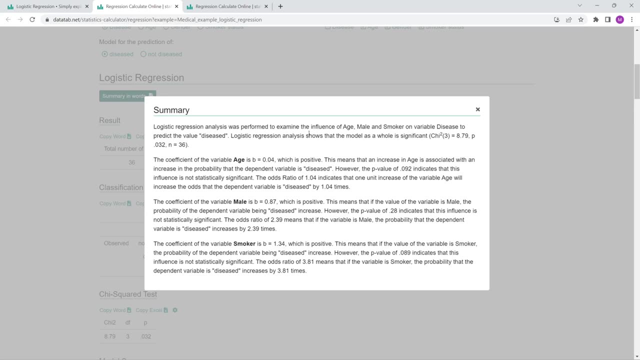 If you don't know how to interpret the results, you can also just click on Summary in words. Logistic regression analysis was performed to examine the influence of age, gender and smoking status as the dependent variables- male and smoker- on variable deceased, to predict the value deceased. 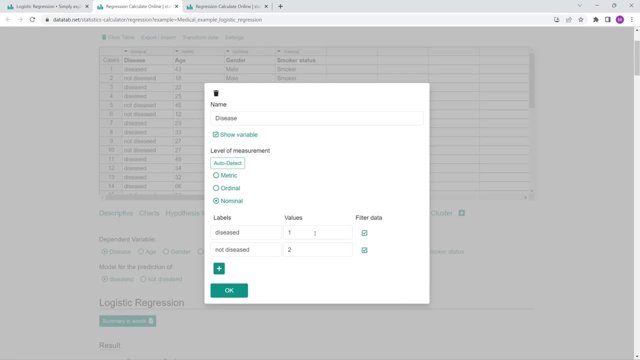 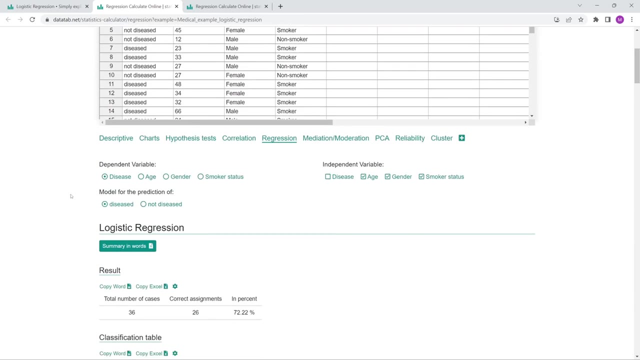 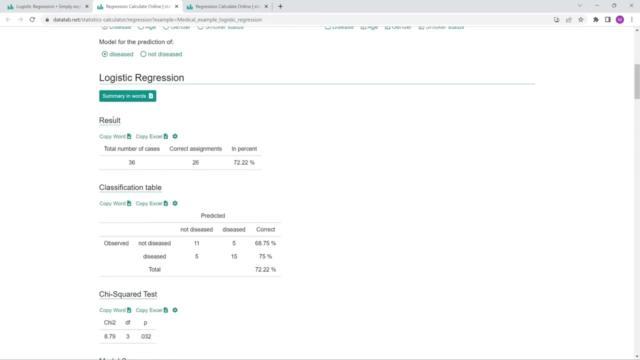 Then we would just need to click here and enter the labels One is deceased and zero is not deceased. Before we go into detail about the different results, a little tip: If you don't know how to interpret the results, you can also just click on Summary in Words. 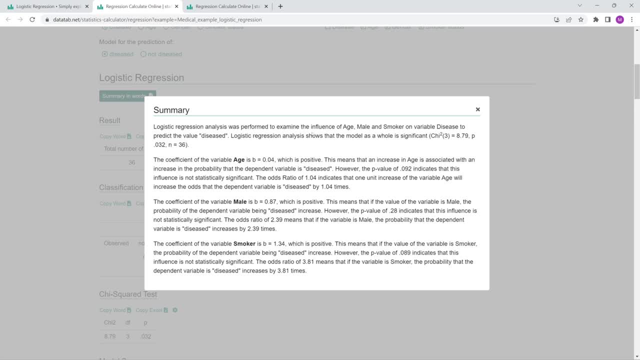 Logistic regression analysis was performed to examine the influence of age, male and smoker on variable disease. to predict the value deceased. Logistic regression analysis shows that the model as a whole is significant. And then come the different independent variables, for example for smokers. 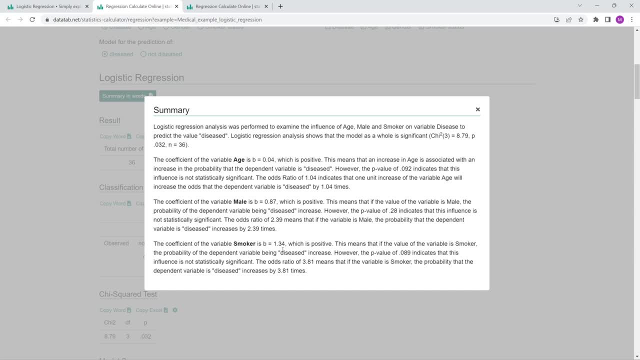 The coefficient of the variable smoker is b equal to 1.34,, which is positive. This means that if the value of the variable is smoker, the probability of the dependent variable being deceased increases. However, the p-value of 0.089 indicates that this influence is not statistically significant. 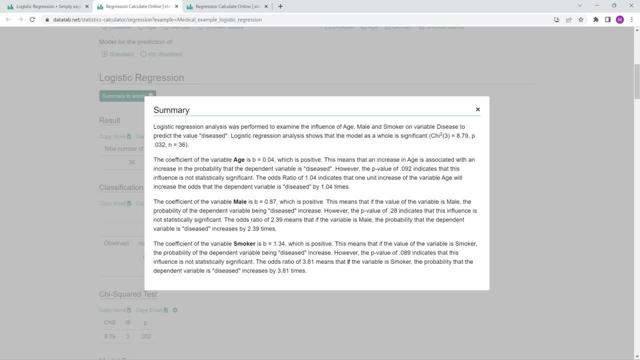 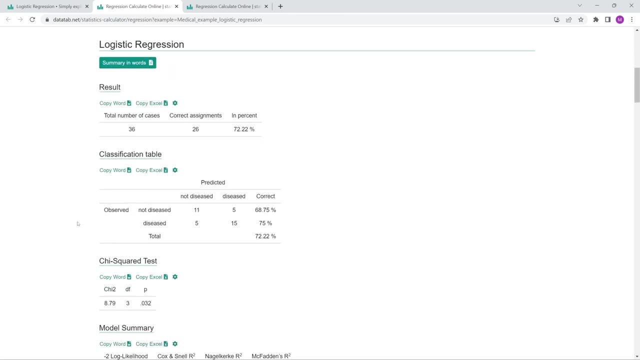 The Oz-ratio of 3.81 means that if the value is smoker, the probability that the dependent variable is deceased increases by 3.81.. But now, in detail, to the results. We will now go through all the tables slowly and understandably. 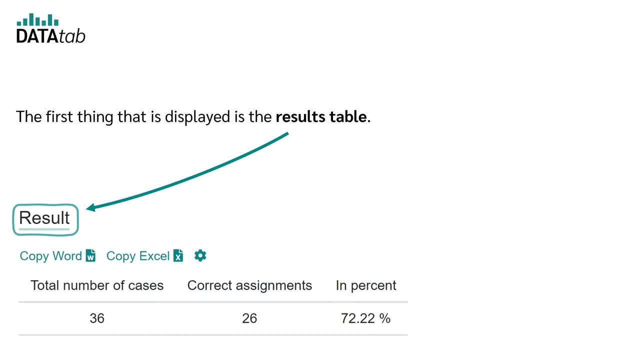 Let's start at the top. The first thing that is displayed is the results table. In the results table, you can see that a total of 36 people were examined. With the help of the calculated regression model, 26 of 36 persons could be correctly. 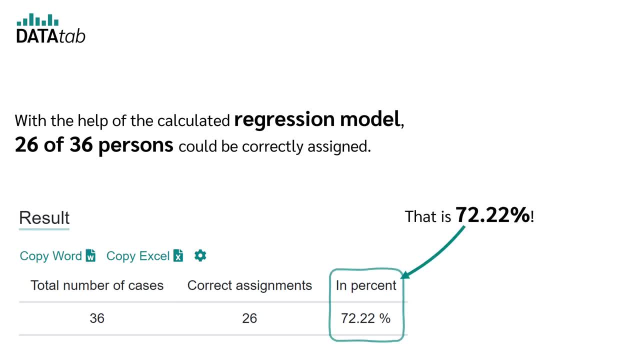 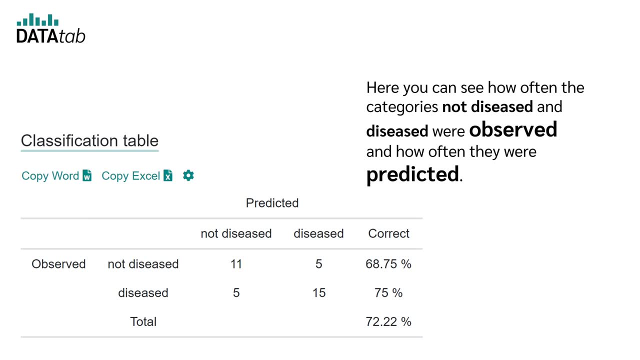 assigned, That is 72.22%. Then comes the classification table. Here you can see how often the categories not deceased and deceased were observed and how often they were predicted. In total, not deceased was observed 16 times. Of these 16 individuals, the regression model correctly scored 11 as not deceased and incorrectly. 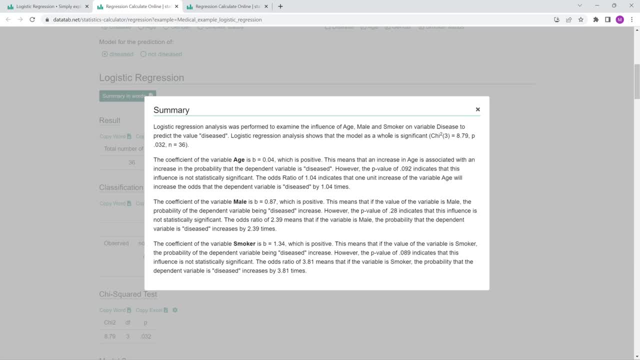 Logistic regression analysis shows that the model as a whole is significant. And then come the different independent variables. for example, for smokers, The coefficient of the variable smoker is b equal to 1.34,, which is positive. This means that if the value of the variable is smoker, the probability of the dependent 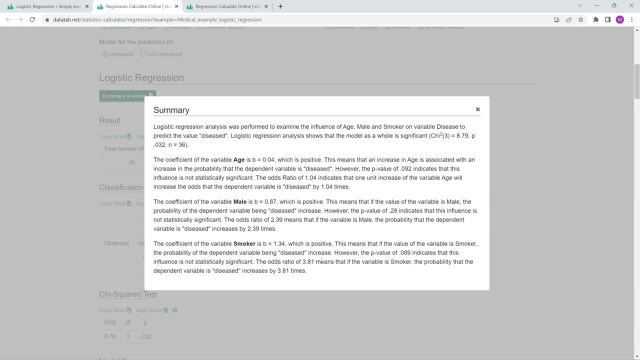 variable being deceased increases. However, the p-value of 0.089 indicates that this influence is not statistically significant. The Oz-ratio of 3.81 means that if the value is smoker, the probability that the dependent variable is deceased increases. 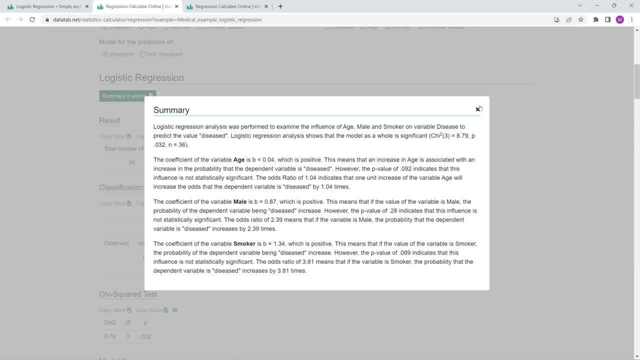 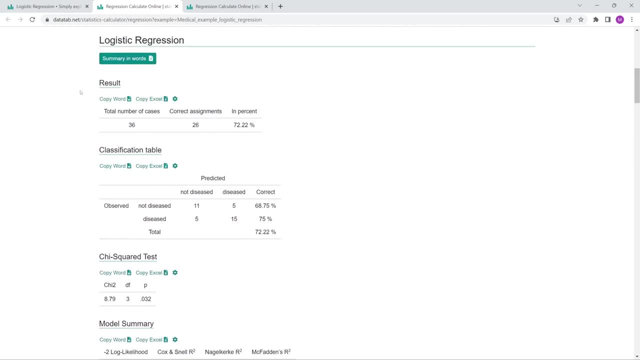 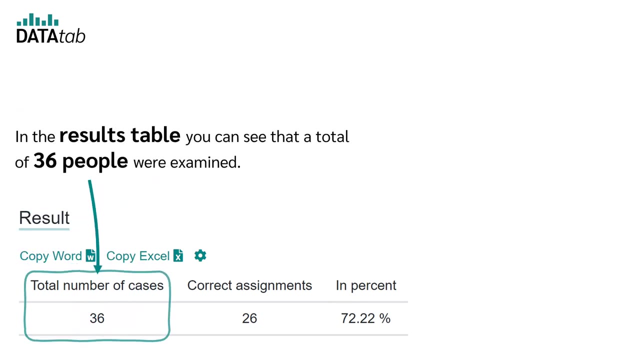 So we can simplify 3.81 times. But now, in detail, to the results. We will now go through all the tables slowly and understandably. Let's start at the top. The first thing that is displayed is the results table. In the results table you can see that a total of 36 people were examined. 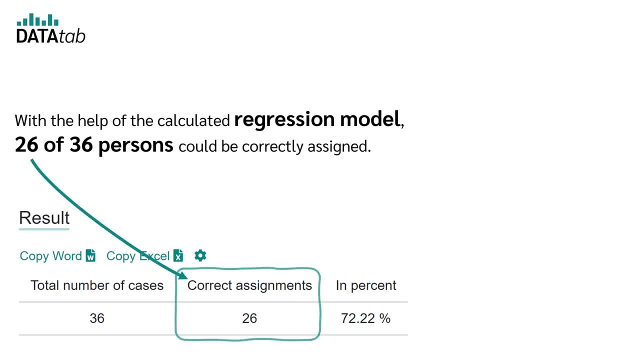 With the help of the calculated regression model, 26 of 36 persons could be correct in the results table. That is, 72.22% of the people were observed as not-deceased and not-deceased as not-deceased. Then comes the classification table. 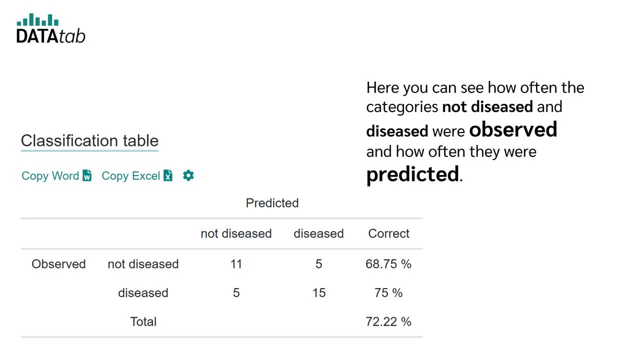 Here you can see how often the categories not-deceased and deceased were observed and how often they were predicted. In total, not-deceased was observed 16 times. Of these 16 individuals, the regression model correctly scored 11 as not-deceased and 16. 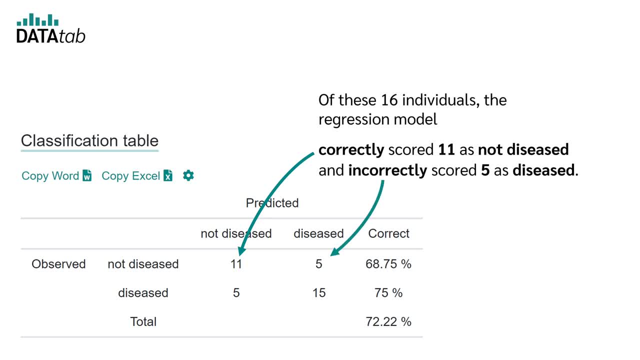 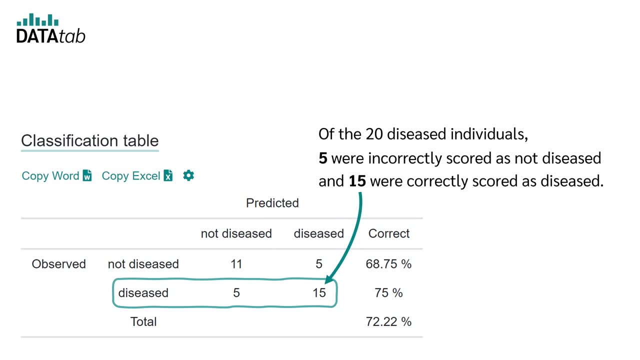 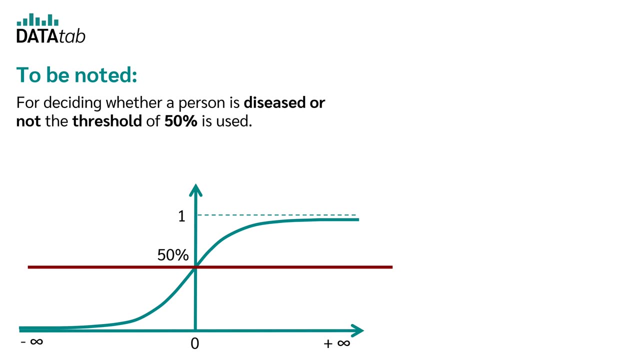 as not-deceased and incorrectly scored 5 as deceased. Of the 20 deceased individuals, 5 were incorrectly scored as not-deceased and 15 were correctly scored as deceased. To be noted for deciding whether a person is deceased or not, the threshold of 50% is: 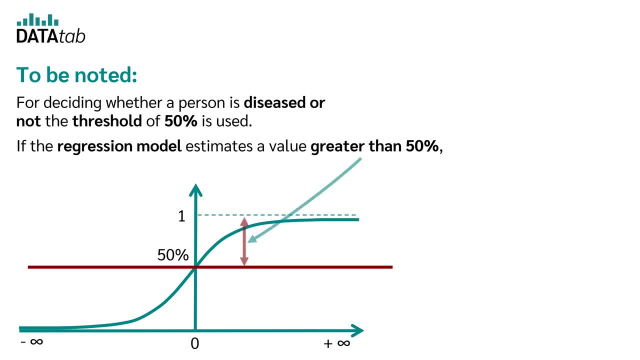 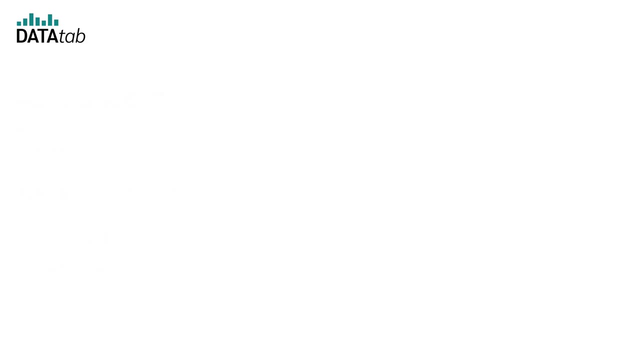 used. If the regression model estimates a value greater than 50%, this person is assigned as deceased, otherwise not-deceased. Now comes the chi-square test. Here we can read whether the model is significant or not. Two models are compared for this purpose. 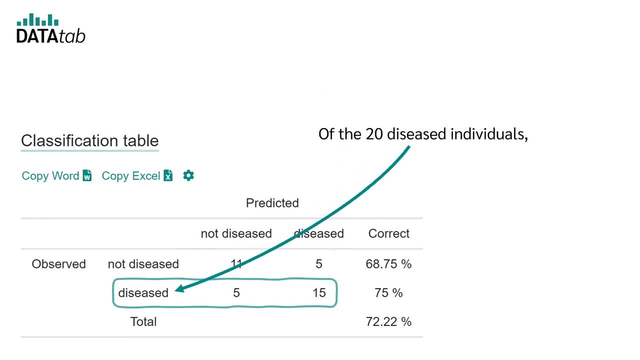 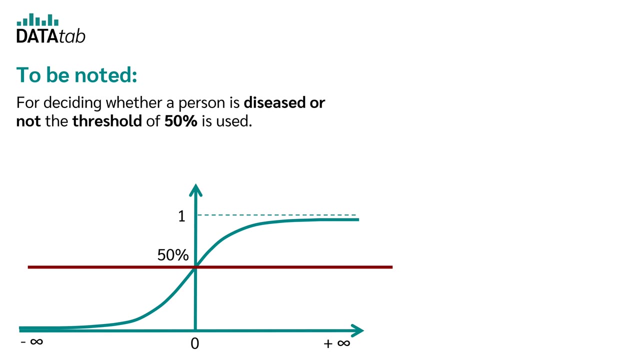 scored 5 as deceased. Of the 20 deceased individuals, 5 were incorrectly scored as not deceased and 15 were correctly scored as deceased. To be noted for deciding whether a person is deceased or not, the threshold of 50% is: 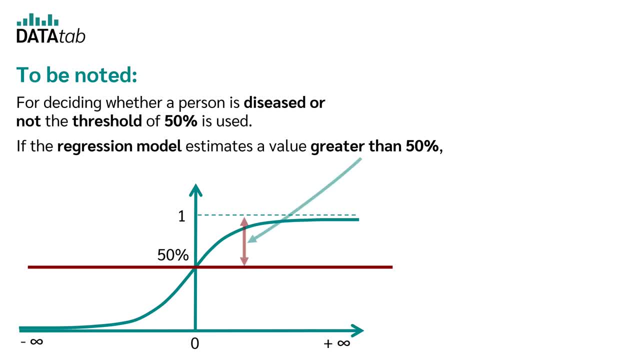 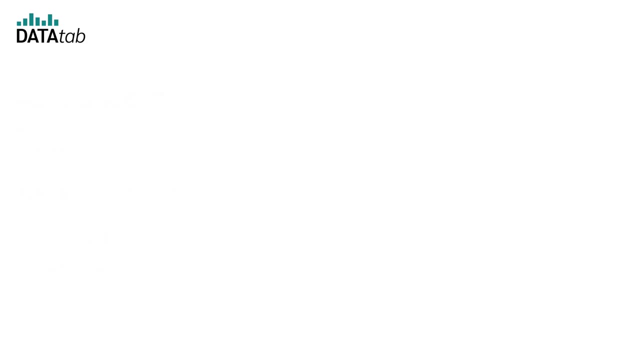 used. If the regression model estimates a value greater than 50%, this person is assigned deceased, Otherwise not deceased. Now comes the chi-square test. Here we can read whether the model is significant or not. Two models are compared for this purpose. 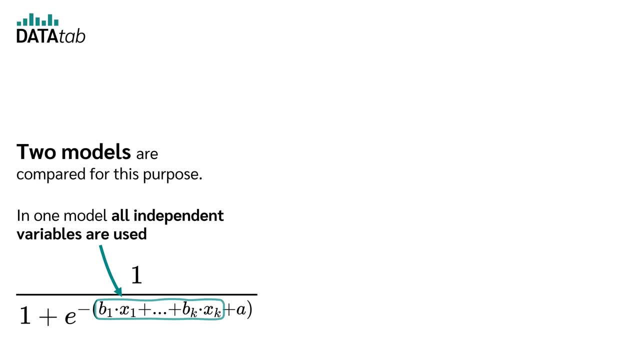 In one model all independent variables are used and in the other model the independent variables are not used. Now we compare how good the prediction is when the dependent variables are used and how good it is when a dependent variable does not. Let's compare this publication window for depetition assessment. 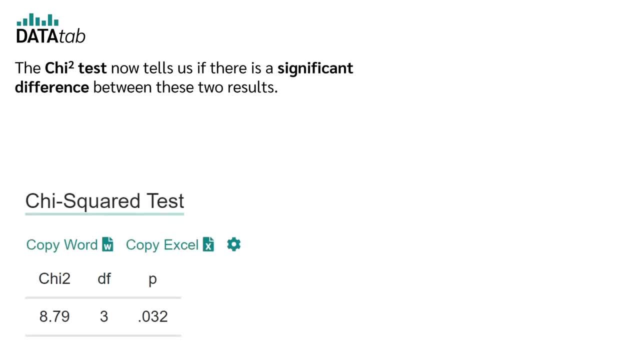 major negligent: 25%, when the dependent variables are not used. The chi-square test now tells us if there is a significant difference between these two results. The null hypothesis is that both models are the same. If the p-value is less than 0.05,, this null hypothesis is rejected. 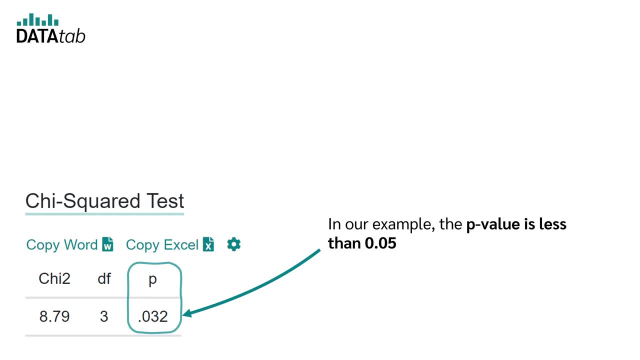 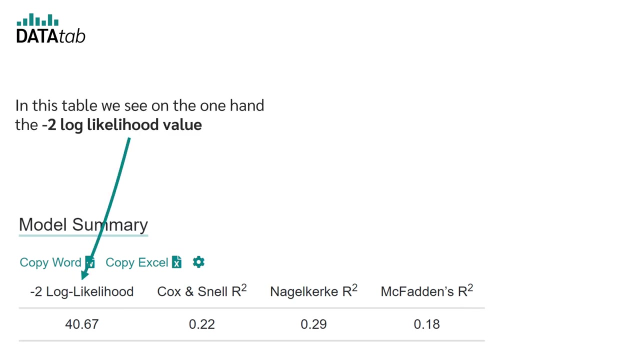 In our example, the p-value is less than 0.05 and we assume that there is a significant difference between the models. Thus the model as a whole is significant. Next comes the model summary. In this table we see on the one hand the minus 2 log-likelihood value and on the other, 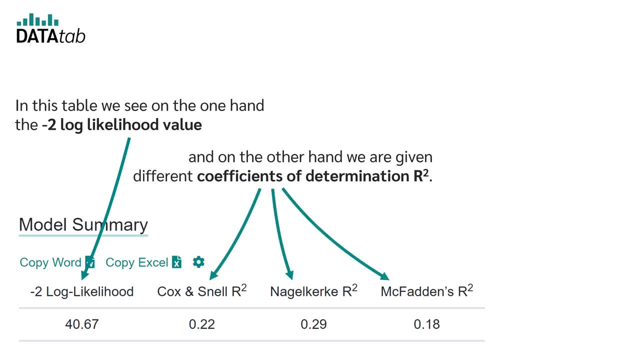 hand, we are given different coefficients of determination: r-square. R-square is the number of coefficients that are equal to r-square. r-square is the number of coefficients that are equal to r-square. r-square is the number of coefficients that are equal to r-square. 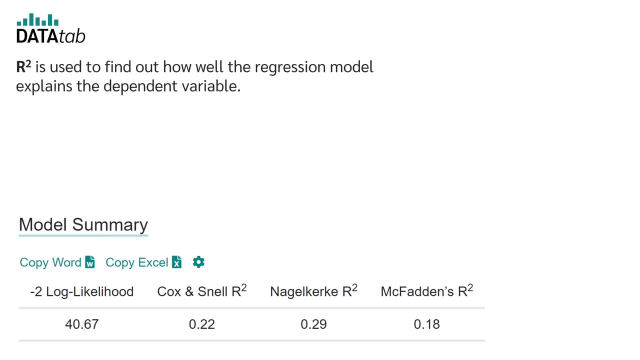 r-square is used to find out how well the regression model explains the dependent variable. In a linear regression, the r-square indicates the proportion of the variance that can be explained by the independent variables. The more variance can be explained, the better the regression model. 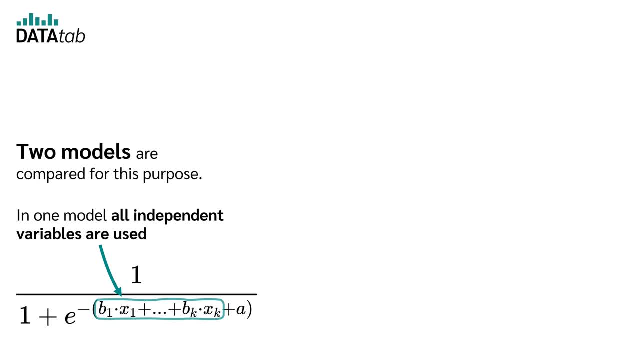 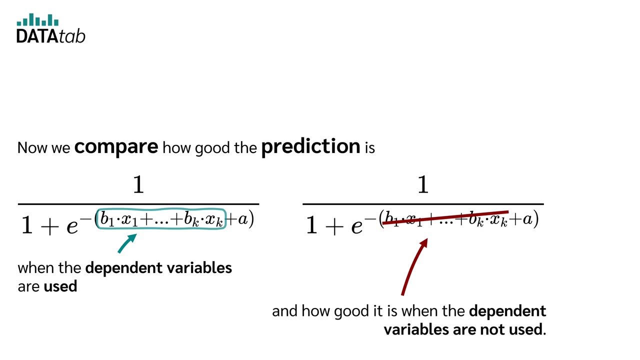 In one model all independent variables are used and in the other model the independent variables are not used. Now we compare how good the prediction is when the dependent variables are used and how good it is when the dependent variables are not used. 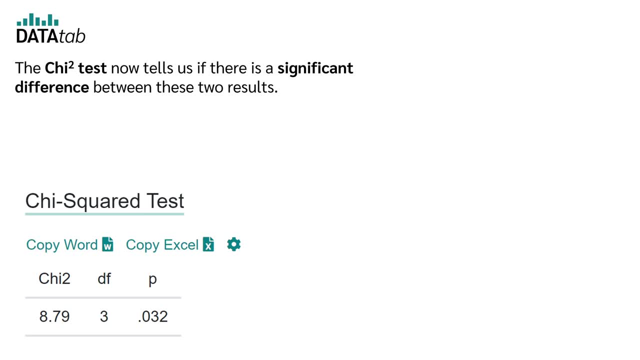 The chi-square test now tells us if there is a significant difference between these two results. The null hypothesis is that both models are the same. If the p-value is less than 0.05, this null hypothesis is rejected. In our example, the p-value is less than 0.05.. 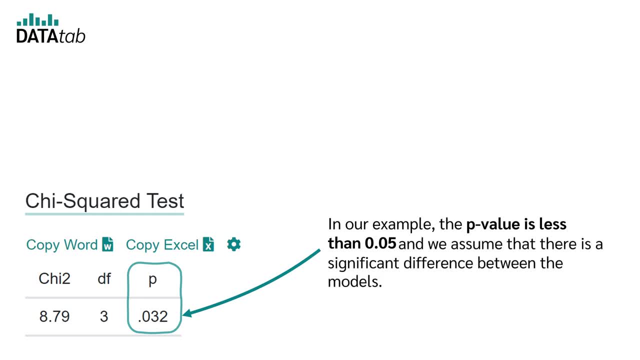 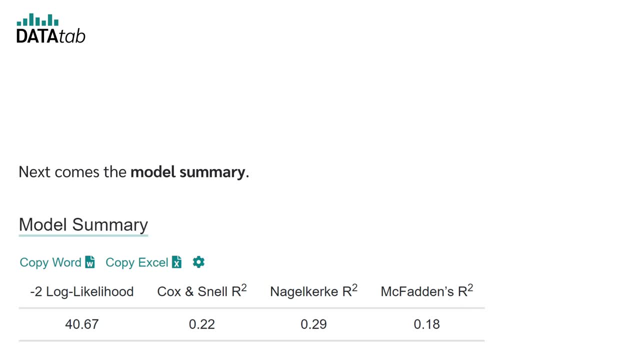 And we assume that there is no difference. The p-value is less than 0.05.. There is a significant difference between the models. Thus the model as a whole is significant. Next comes the model summary. In this table we see on the one hand the minus-two log-likelihood value and on the 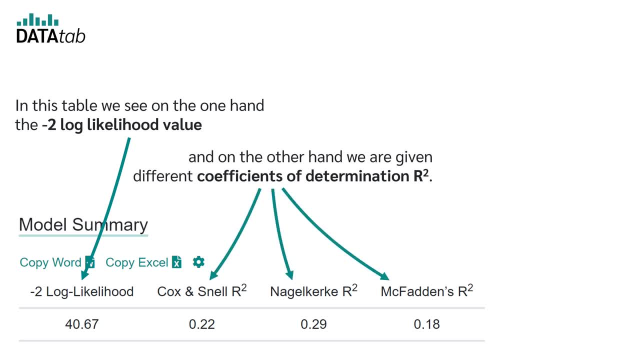 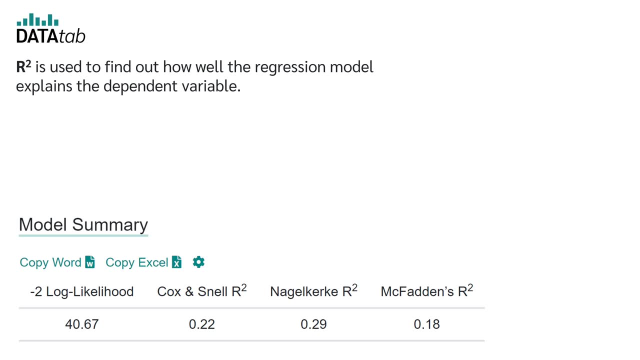 other hand, we are given different coefficients of determination: r-square. R-square is used to find out how well the regression model explains the dependent variable. In a linear regression, the r-square indicates the proportion of the variance that can be explained by the independent variables. 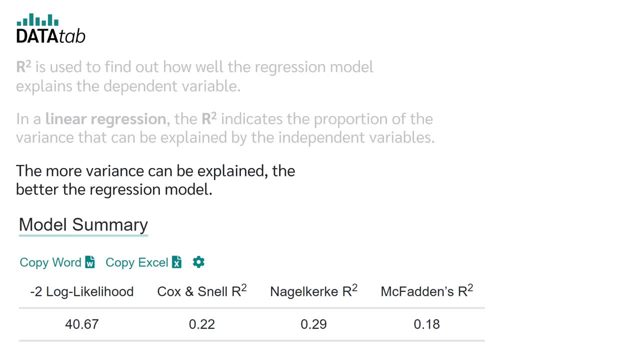 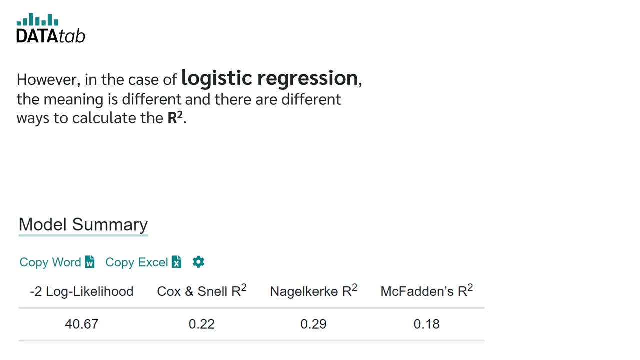 The more variance can be explained, the better the regression model. However, in the case of logistic regression, the meaning is different and there are different ways to calculate the r-square. Unfortunately, there is also no agreement yet on which way is the best way. 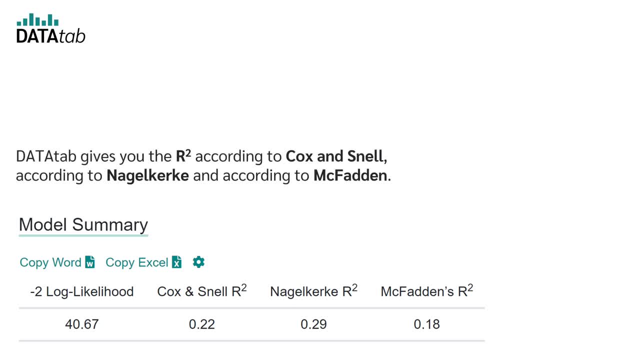 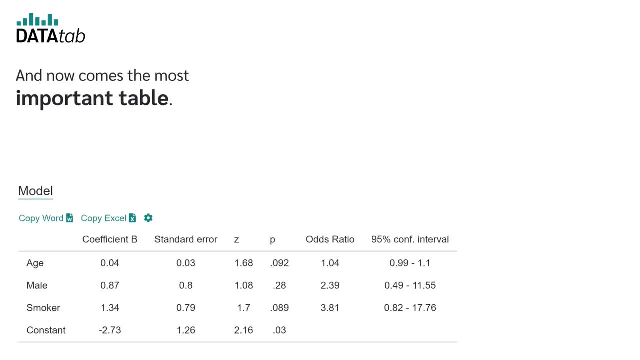 DataDep gives you the r-square according to Cox and Snell, according to Nagel-Kerke and according to McFadden. And now comes the most important table, the table with the model coefficients. The most important parameters are the coefficient b, the p-value and the odds ratio. 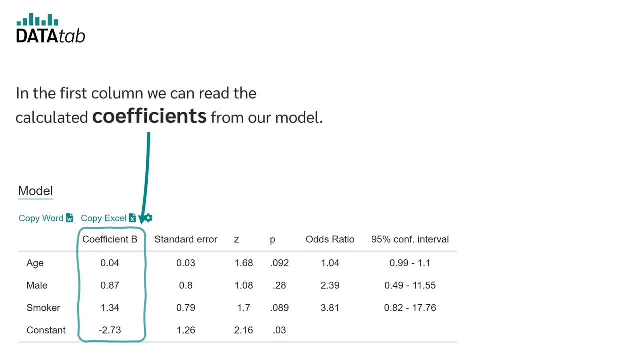 We will now discuss all three columns. In the first column we can read the calculated coefficients from our model. DataDep gives you the r-square according to Cox and Snell, according to Nagel-Kerke and according to McFadden. 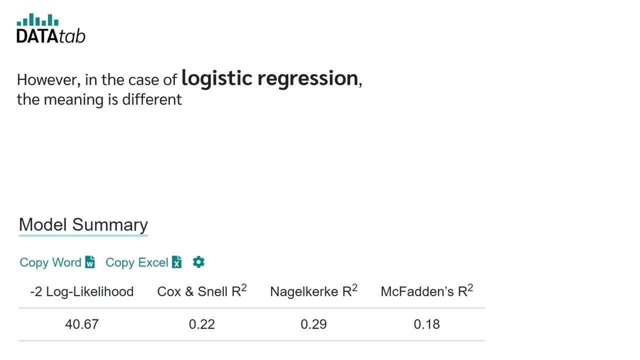 However, in the case of logistic regression, the meaning is different and there are different ways to calculate the r-square. Unfortunately, there is also no agreement yet on which way is the best way? DataDap gives you the r-square, according to Cox and Snell, according to Nagel-Kerke and. 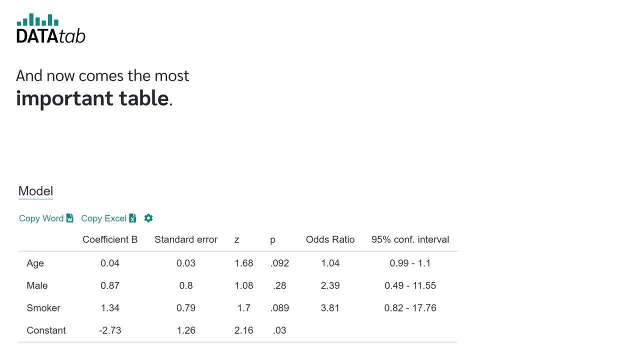 according to McFadden. And now comes the most important table, the table with the model coefficients. The most important parameters are the coefficient b, the p-value and the odds ratio. We will now discuss all three coefficients. In the first column we can read the calculated coefficients from our model. 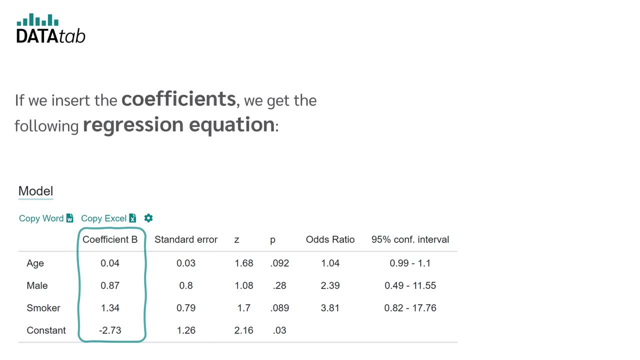 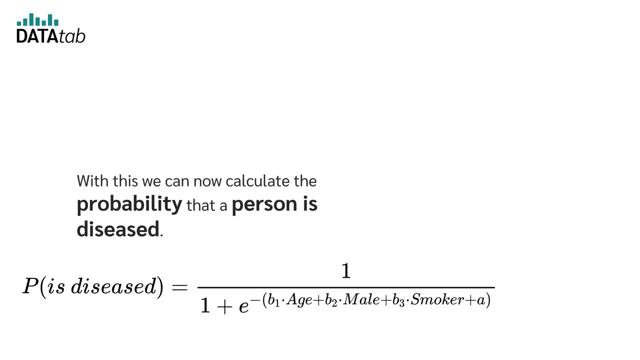 We can insert these into the regression equation. If we insert the coefficients, we get the following regression equation: 0.04, 0.87, 1.34, minus 2.73.. With this we can now calculate the probability that the person is deceased. 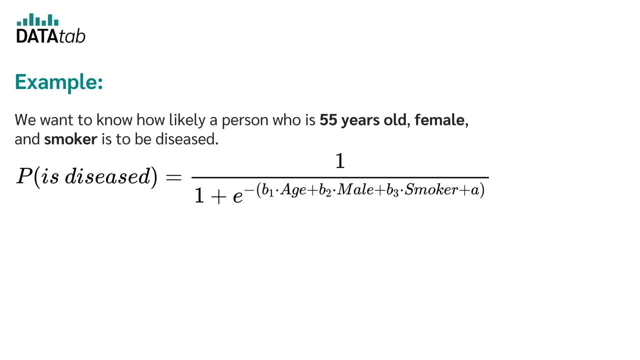 For example, we want to know how likely a person who is 55 years old, female and smoker is to be deceased. We insert 55 for the age, 0 because the person is female and 1 as the person is a smoker. 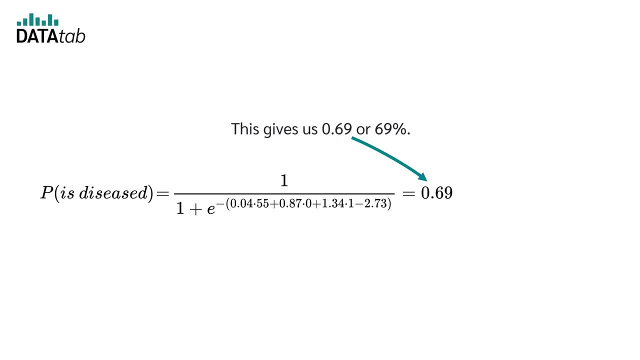 This gives us 0.69 or 69%. Thus, it is 69% likely that a 55-year-old person is a smoker. We can now calculate the probability of a person being a smoker. We can now calculate the probability of a person being a smoker. 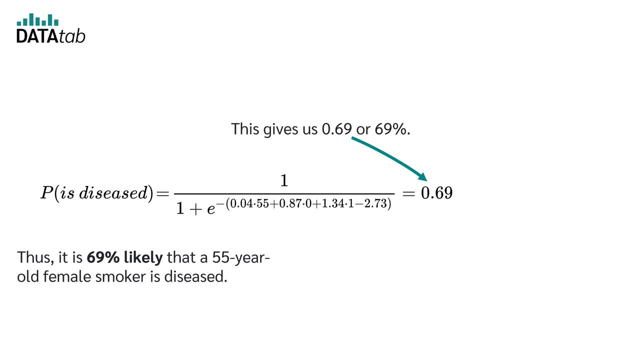 We can now calculate the probability of a person being a smoker. Therefore, we can calculate the probability that a 55 year old female smoker is deceased. Based on this prediction, it could now be decided whether to do another extensive investigation. As I said, the example is purely fictitious. 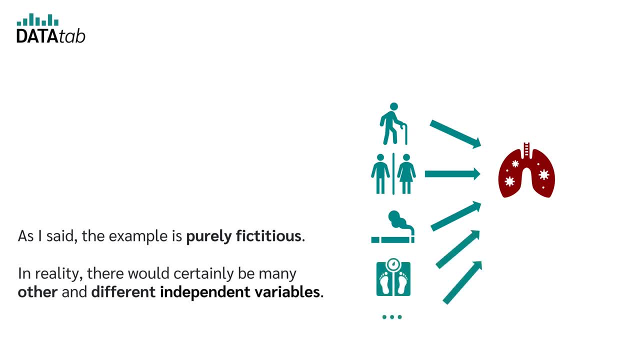 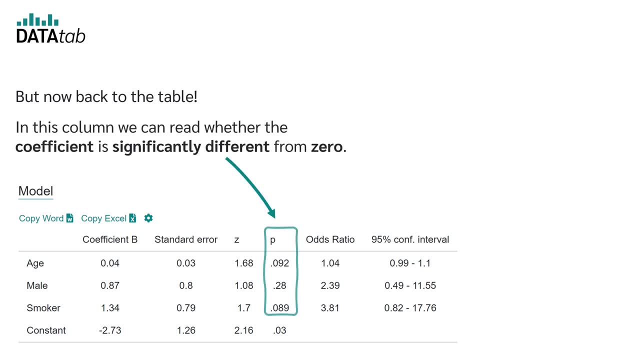 In reality there would certainly be many other and different independent variables. But now back to the table. In this column we can read whether the coefficient is significantly different from 0. Our separating coefficient value is 1.. Let's get back to thisjshar blir effektiv. 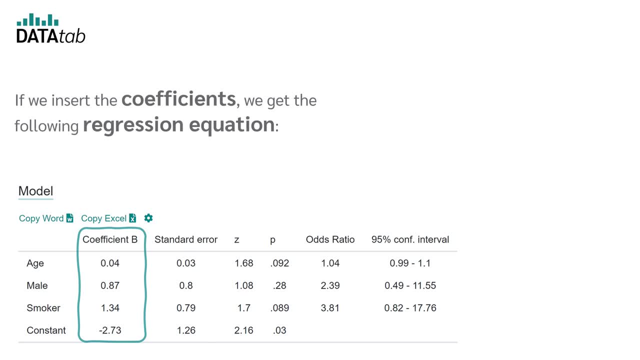 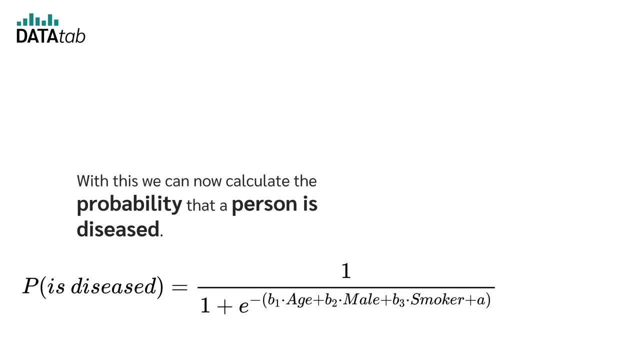 We can insert these into the regression equation. If we insert the coefficients, we get the following regression equation: 0.04, 0.87, 1.34, minus 2.73.. With this we can now calculate the probability that the person is deceased. 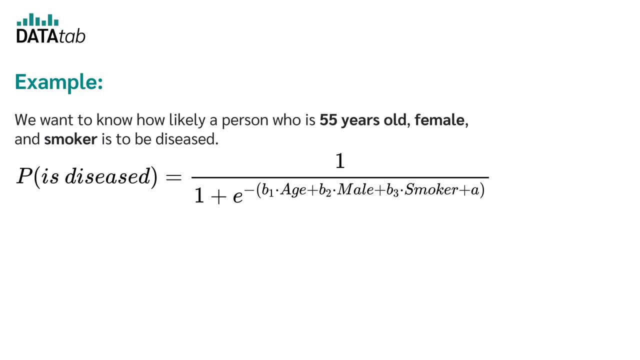 An example. We want to know how likely a person who is 55 years old is to die. A person who is 55 years old, female and smoker is to be deceased. We insert 55 for the age, 0 because the person is female and 1 as the person is a smoker. 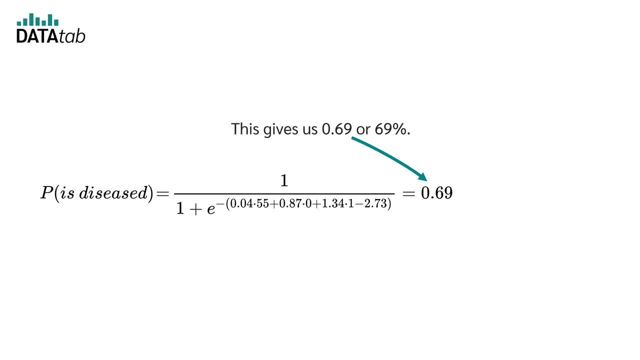 This gives us 0.69 or 69%. Thus, it is 69% likely that a 55-year-old female smoker is deceased. Based on this prediction, it could be said that the person is a smoker. It could now be decided whether to do another extensive investigation. 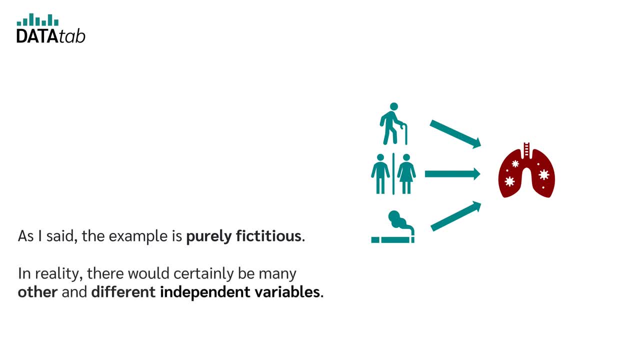 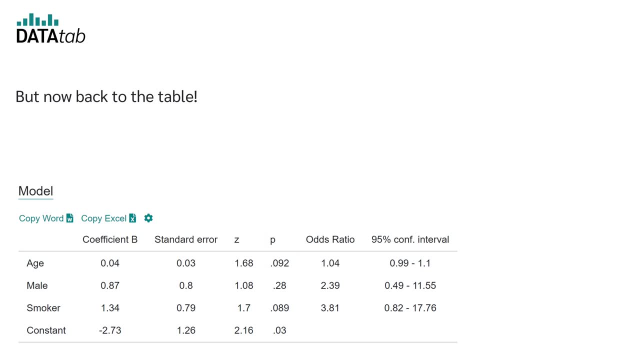 As I said, the example is purely fictitious. In reality there would certainly be many other and different independent variables. But now back to the table. In this column we can read whether the coefficient is significantly different from zero. The following null hypothesis is tested: 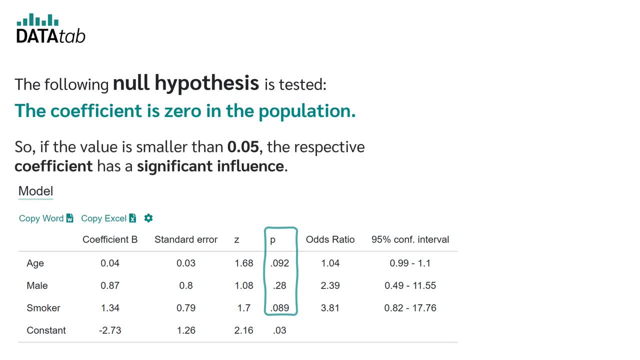 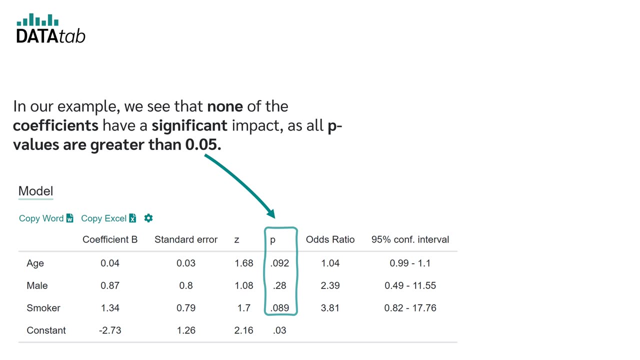 The coefficient is zero in the population. The coefficient is zero in the population, So if the value is smaller than 0.05, the respective coefficient has a significant influence. In our example, we see that none of the coefficients have a significant impact, as all p-values. 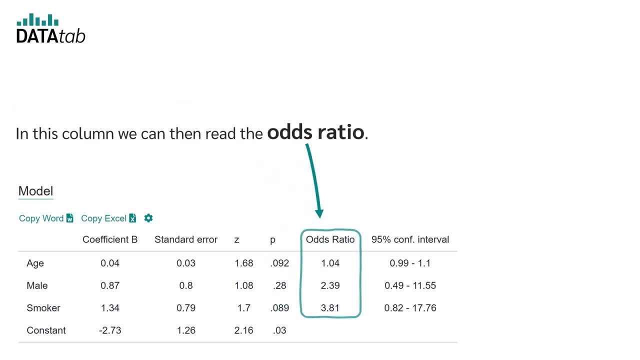 are greater than 0.05.. In this column we can then read the odds ratio. For example, the odds ratio of 1.04 means that a one-unit increase in the population in a variable age, which means that the person is one year older, increases the probability. 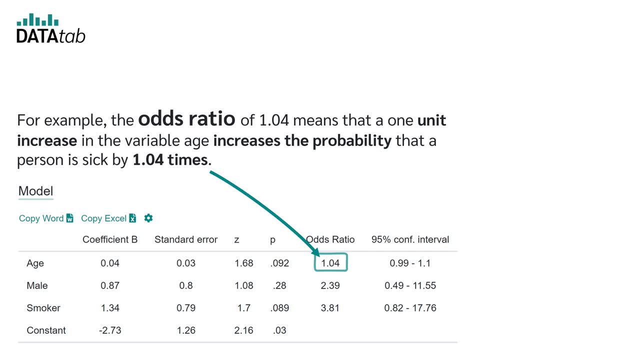 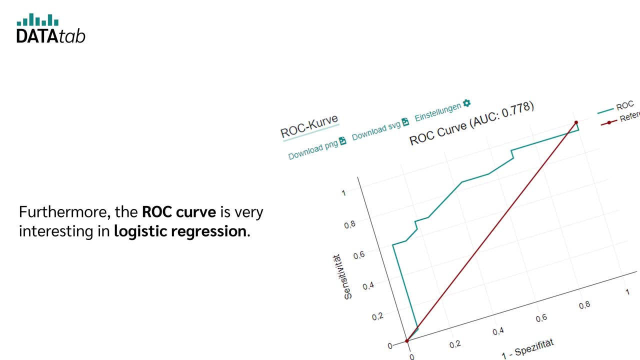 that the person is sick by 1.04 times. Furthermore, the receiver operating characteristic ROC curve is very interesting in logistic regression. If you want to know what the ROC curve is and how to interpret it, watch our video on ROC curve. Thanks for watching and see you next time.